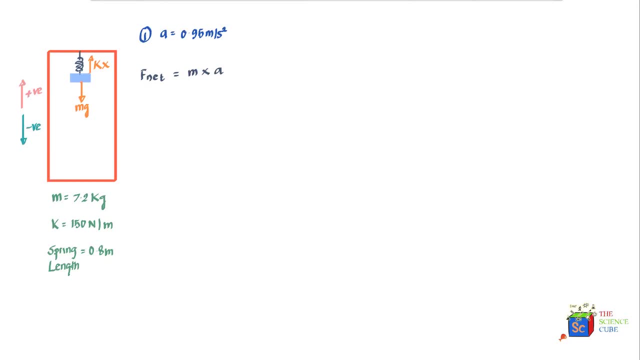 direction as negative. Now, with these rules, let's find what is the net force. To find the net force, we'll put all the forces acting on this mass And the first force we see is force kx acting in upward direction. and it'll be positive because 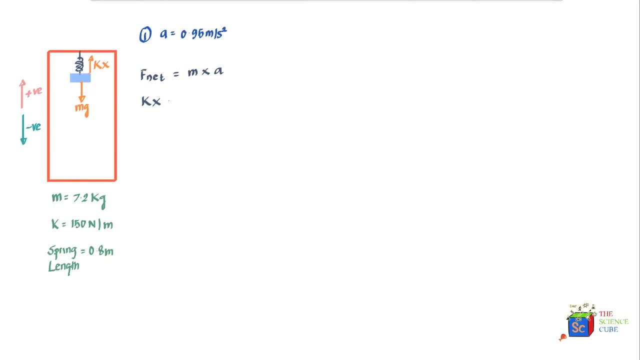 this vector is pointing in upward direction And you have mg pointing in downward direction, so we'll say it's negative and this should equal product of mass and acceleration of the elevator, which is also the acceleration of the mass. Now, one thing you would have noticed here is that 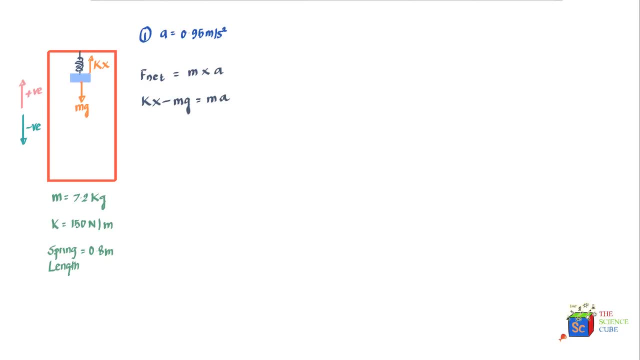 you've taken kx as positive, but in on most occasions what we take is f is equal to minus kx when we deal with springs, And the reason for this is that on most occasions we have a. we have a setup like this, where you have a spring which is attached to a. 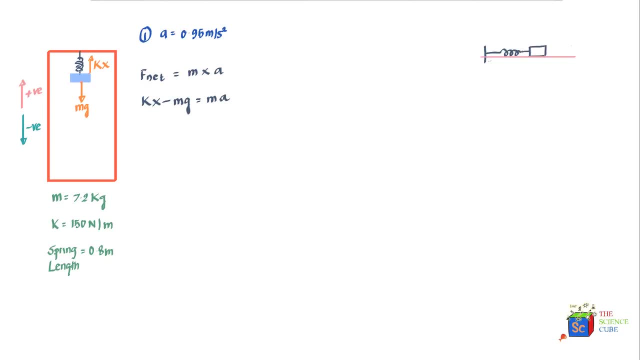 mass and probably it's on a table or something and the mass is pulled in this direction by a distance, x, And the vector notation under this setup very often is that any vector pointing in this direction would be taken as positive and any vector pointing in downward direction would be positive. 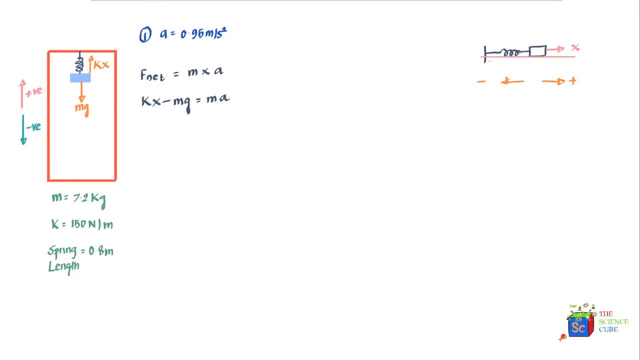 And when you pull it by a distance- x- it's a positive vector. the displacement vector is positive and therefore we say f is equal to minus kx, because the force is acting in this direction, the pull of the string is in this direction and therefore if x is positive, the negative sign here: 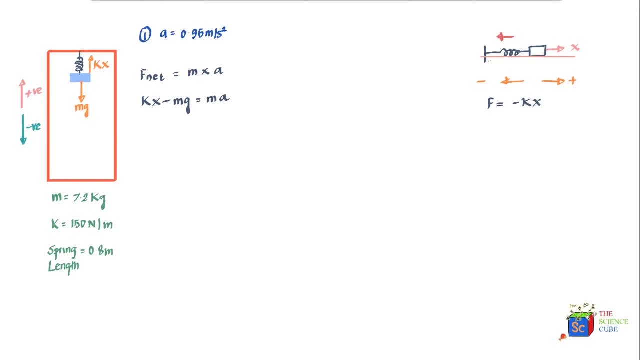 connotes that the force is acting in reverse direction. However, you see, in this setup, because the sign notation we've taken, kx is positive because it's pointing in upward direction, So you see that the sign we take for denoting the vectors plays a big role in how our equations shape. 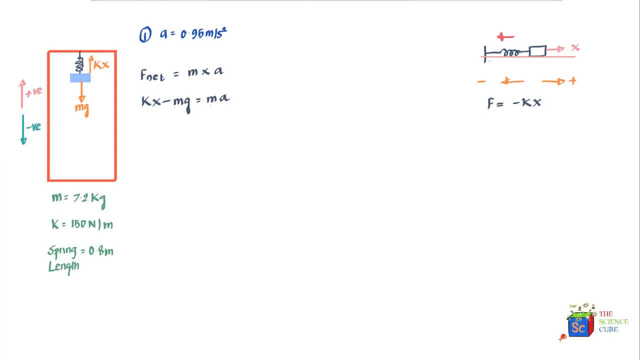 up. So, getting back to this equation, we have derived force kx is acting in upward direction, mg is acting in downward direction and therefore negative, and this is equal to mass into acceleration, and acceleration here would be positive because the elevator is moving in upward direction and any vector in upward direction is positive. So in a way this a value here. 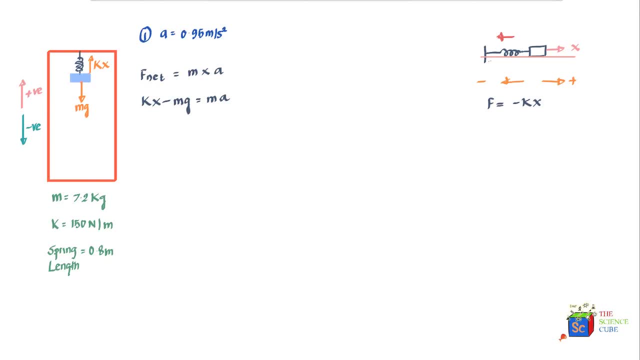 is the absolute value because the sign has been taken into account. So if we have this equation, you'll find that x equals m into g, plus a upon k, and if we substitute the values which we have available, what we find is x is equal to seven point two kilograms multiplied by nine point. 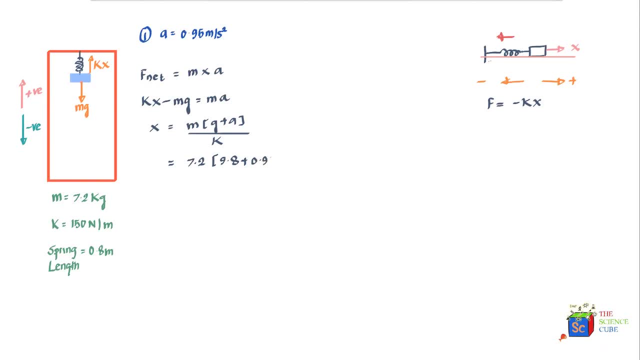 eight plus zero point nine, five meters per second square divided by one hundred fifty newton per meter, and what you get is zero point five, two meters. So the stretch that the mass would experience when the lift moves up with an acceleration of 0.95 meters per second square. 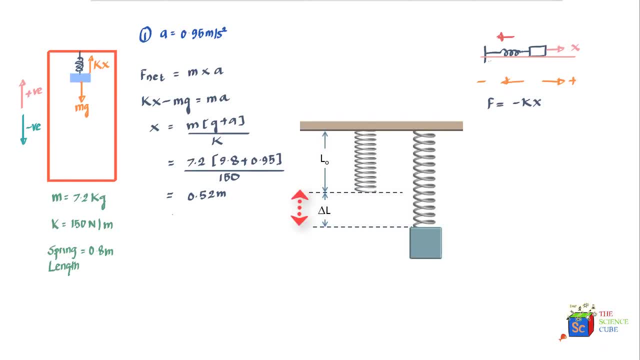 would be 0.52 meters, or the length of the spring would therefore be zero point. eight meters plus 0.52 meters. Now the second question is: what is the stretch in the spring if the elevator is moving up with a constant velocity of 14 meters per second, that is, it has accelerated? 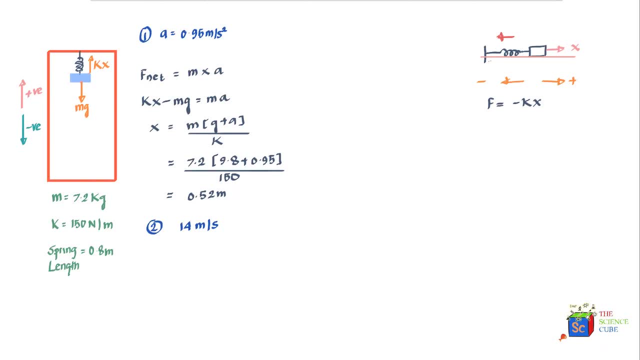 up, and then it has stopped accelerating and it's now moving up with a constant velocity of 14 meters per second. So what you would understand is that the forces acting on the mass continue to be the same, That is, kx acts in upward direction, mg acts in downward direction, and this should equal to the 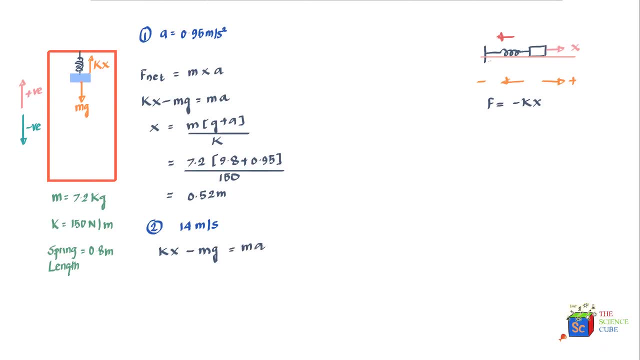 product of mass and acceleration. But the problem says that now the elevator is moving up at a constant velocity, that is, the acceleration is zero and therefore kx should equal mg or x should equal mg upon k, and if you substitute the value of g and k, what you get is x equals 0.47 meters. Now the third part of the problem is- and let me go- 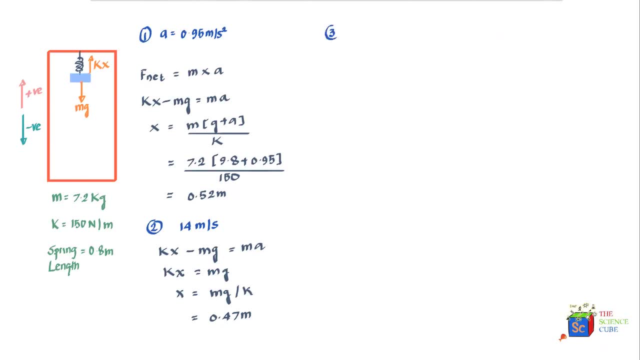 ahead and rub off this portion. the third part of the problem is: what is the stretch in the spring if the elevator reduces its velocity from 14 meters per second to zero meters per second in nine seconds? So what we'll do is we'll find what is the deceleration of the elevator and and we know the deceleration- 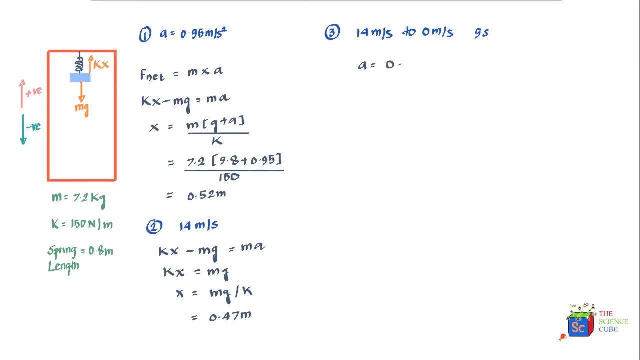 would equal to the final velocity, which is 0 minus 14 meters per second, which was the initial velocity divided by the time taken. and what we find is this is equal to minus 1.5 meters per second squared. So once again, let's write Newton's second law of motion equation and see what. 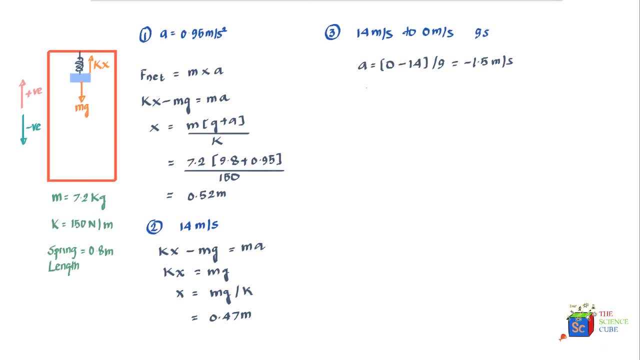 are the forces acting on the mass. We know one force is kx acting in upward direction, mg acting in downward direction, and this should equal to the product of mass and acceleration. and once again we solve for x, which is m into g, plus a upon k. and if we substitute the 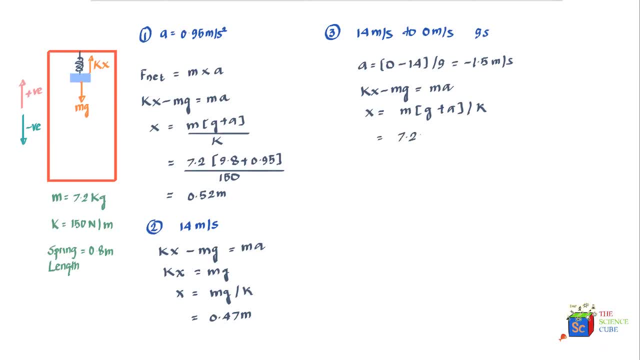 values. what we get is m is 7.2 kilograms into 9.8 and, as we said, a here is absolute value. that is a sign has been taken care of. We'll just go ahead and substitute minus 1.5 meters per second squared divided by 150. 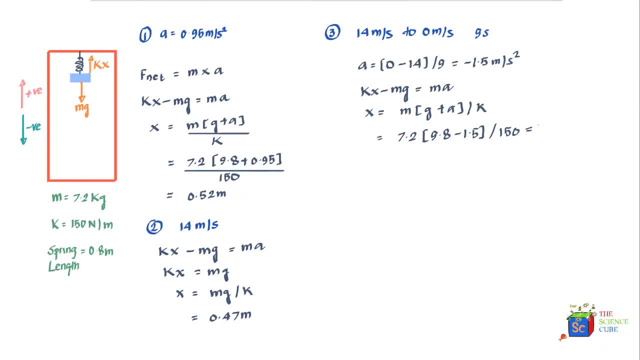 which you'll find is equal to 0.4 meters. Now, what you would have observed is that first the stretch was 0.52, then it reduced to 0.47 and then it further reduced to 0.4 meter. Now, the reason for this is that initially, when the elevator was 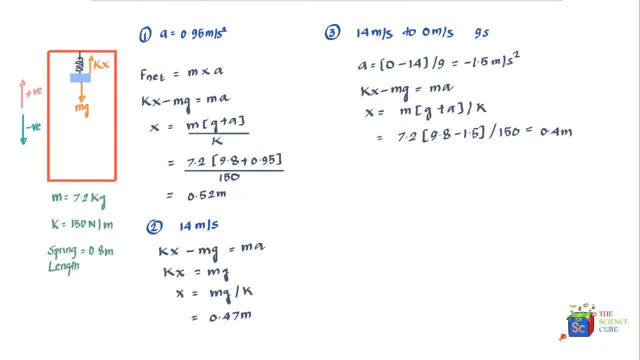 accelerating. we have learned in the earlier lesson that a mass experiences increase in weight as the elevator accelerates, and that's a reason that the spring is stretched by 52 centimeter. a larger stretch in the spring indicates a larger weight and then, when the velocity steady, it's the stretch. 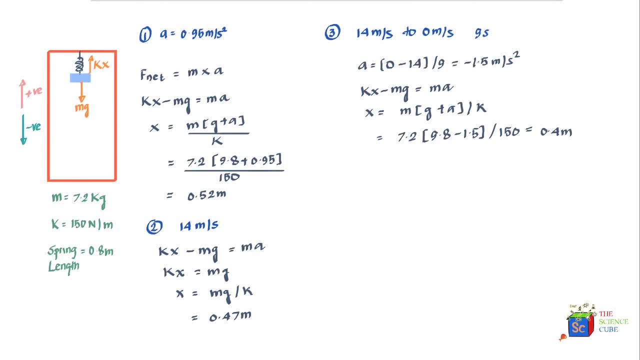 in the spring was 0.47 meters, that is, it was not experiencing any gain in weight or loss in weight. in fact, this weight is the same as the weight would be if the elevator was stationary. so constant velocity of the elevator and the elevator being stationary, you'll get a similar 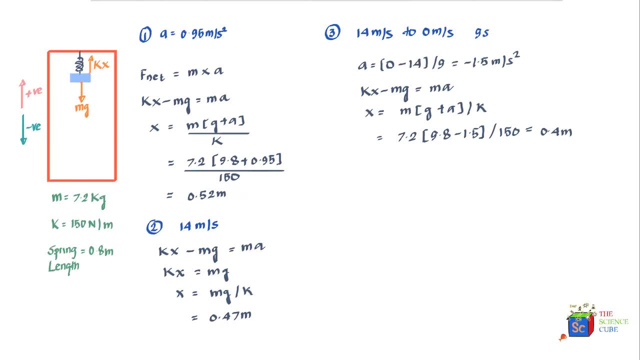 weight and when, finally, the elevator decelerates, all bodies inside the elevator would experience a loss in weight, and that's a reason the stretch of the spring is further reduced to 0.4 meters, because it's indicating that there's a lesser stretch in the spring.